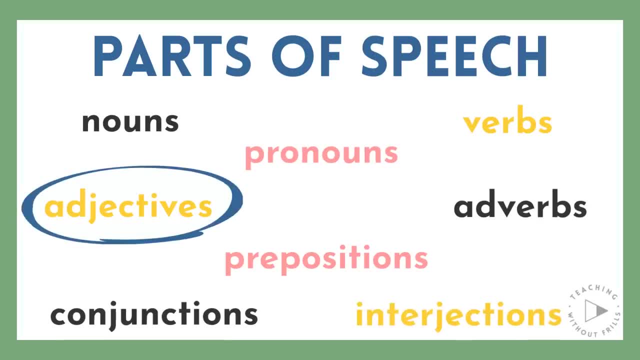 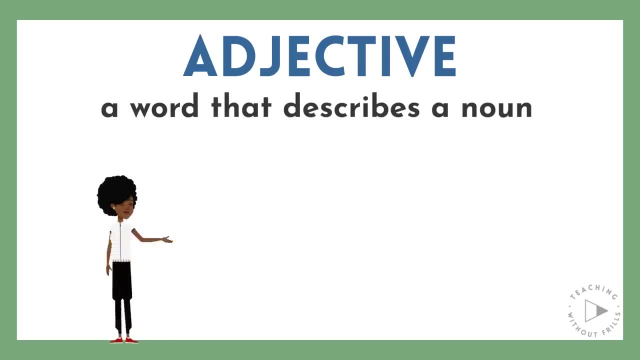 and interjections. So what's an adjective? An adjective is a word that describes a noun. A noun is a person, place or thing. Adjectives tell details about nouns, like a friendly woman, a tall building, a furry bear. Friendly, tall and furry are all adjectives. 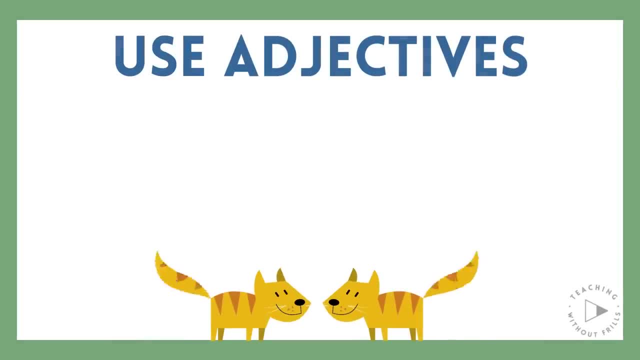 Can you use adjectives? Can you use adjectives to describe these cats? Pause here to think or keep watching. Adjectives can describe how something looks, so you might have said orange or cute. Adjectives can also describe how something feels, so maybe you said soft. 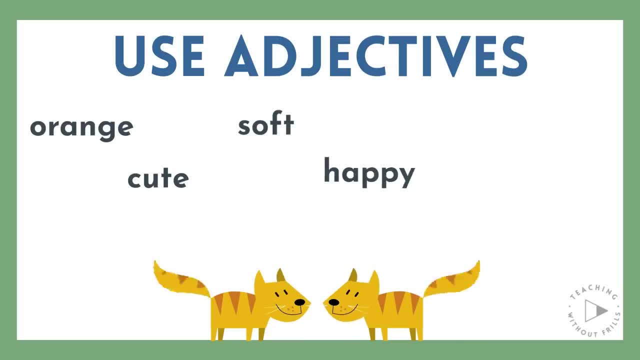 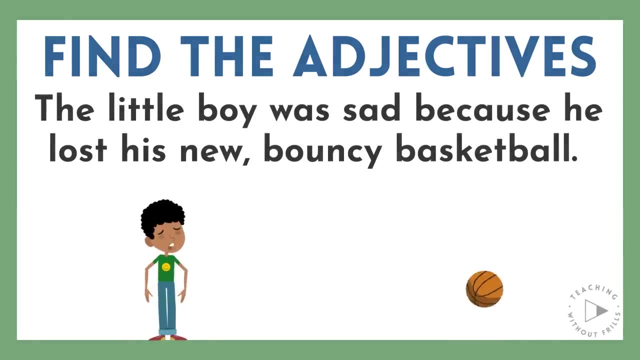 They can also tell how something acts like happy or nice. Adjectives can even tell how many, so two is an adjective also. now can you find the adjectives in the following sentence. the little boy was sad because he lost his new bouncy basketball. here's a hint: there are four adjectives in this sentence. 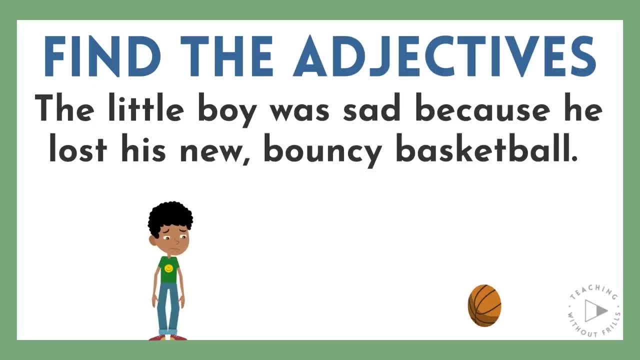 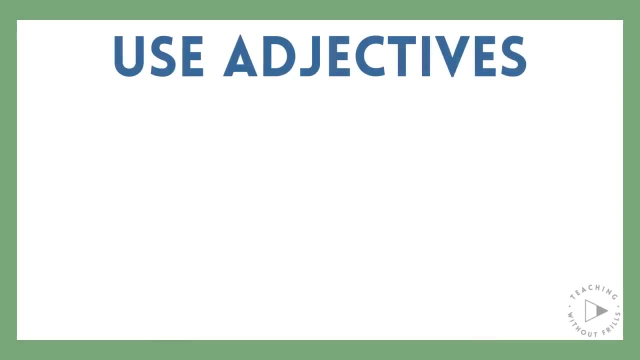 pause here to think or keep watching to hear the answer. little and sad are adjectives that describe the boy. new and bouncy are adjectives that describe the basketball. so how can you use adjectives? listen to this boring sentence: the bees flew around the flowers. how can you add some describing words to this sentence to make? 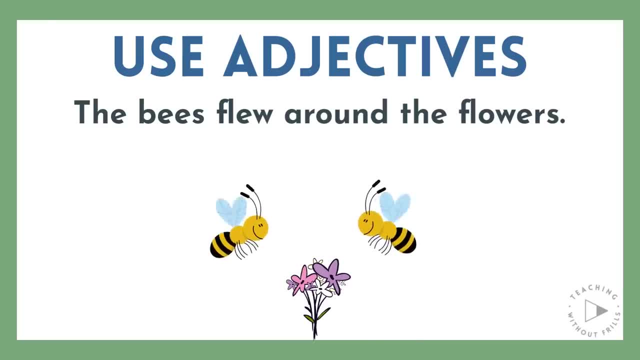 it more detailed and interesting. pause here to think or keep watching. there are many ways you could add adjectives to this sentence. you might say: the two bees flew around the colorful flowers, or maybe the happy bees flew around the pretty flowers. So remember, adjectives are words we use to describe nouns. You can use: 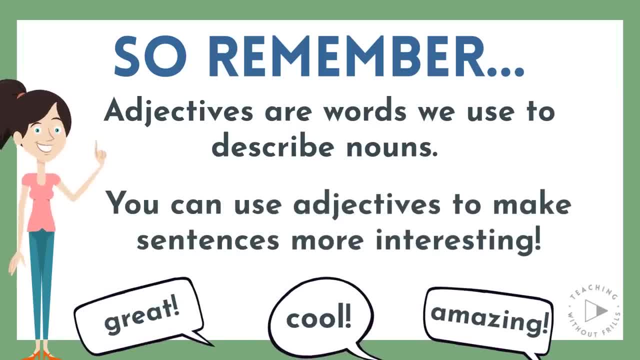 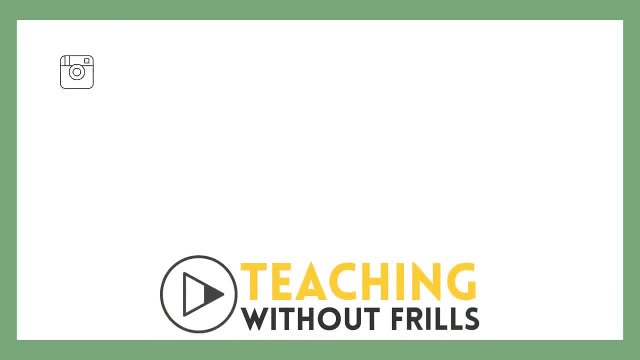 adjectives to make sentences more interesting. Check out the other videos in this series to learn more about different parts of speech. If you're a teacher, you can find Teaching Without Frills on Instagram, Facebook, Pinterest and TPT for related resources. Thanks for watching.